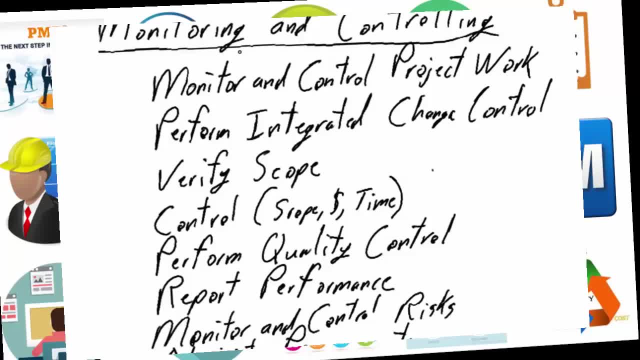 execution. that's where the project team spends the most of their time delivering the project. While the team is busy in executing delivering the project, we, the project managers, are busy in monitoring and controlling the project. The main activity in monitoring and controlling from our integration knowledge area, is monitoring. 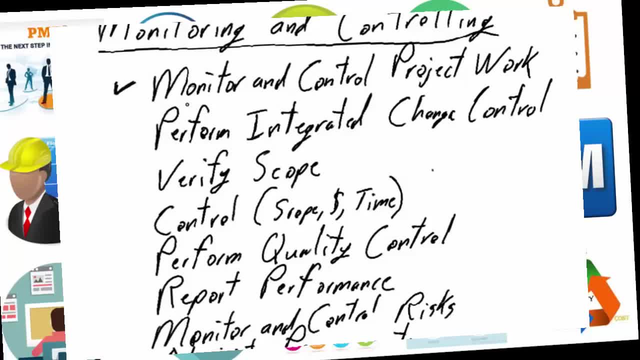 and controlling the project work. Making sure all of the bits and pieces, make sure the schedule, the time, the cost, the quality. making sure that each and every one of our nine knowledge areas are being properly implemented on our project. Monitoring and control of project work much. 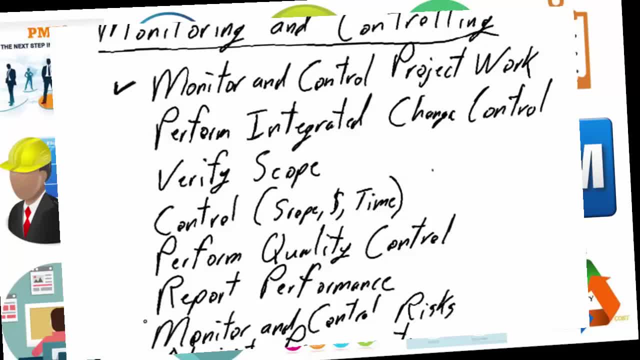 like we saw in executing, is really best defined through the remaining processes. Perform integrated change control, Making sure that all- can- I say all 36 times and not bore you- ensuring that all changes are properly processed and documented through integrated change control and that changes are integrated, That when we're looking at a change we just don't say. 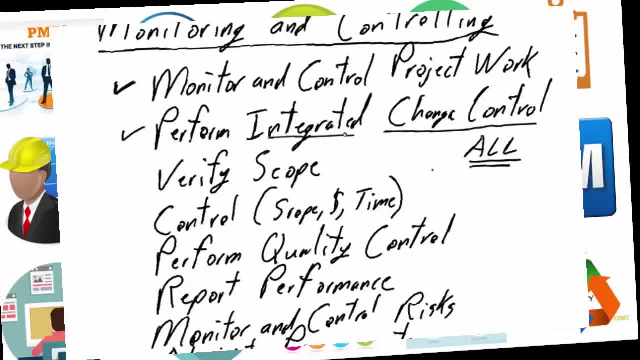 oh, that affects the budget or that affects the cost. That we look at the impact of all changes for scope, for time, for cost, for human resources, for procurement, for risk, for quality and so on. that we ensure that all changes are fully integrated across all. 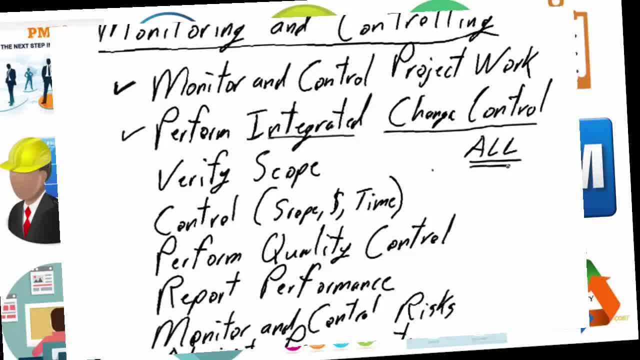 of the knowledge areas and that all changes are, in fact, addressed and documented through monitoring and control. Monitoring and Control is all about verifying the scope. As we said in the scope nuggets. verifying the scope is not related to integrated change control and ensuring you're only doing the scope work. verifying the scope is focused on 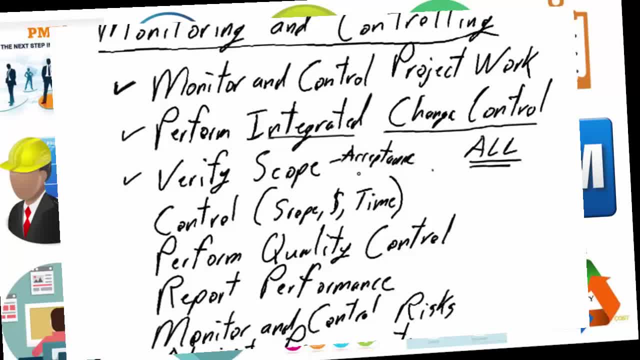 acceptance. ensuring that the work, ensuring that the quality of the work, ensuring that the focus of the work, ensuring that the the depth and breadth of the work being done is focused on acceptance. validating that all of the deliverables will meet the project requirements. verifying the scopes. it's. 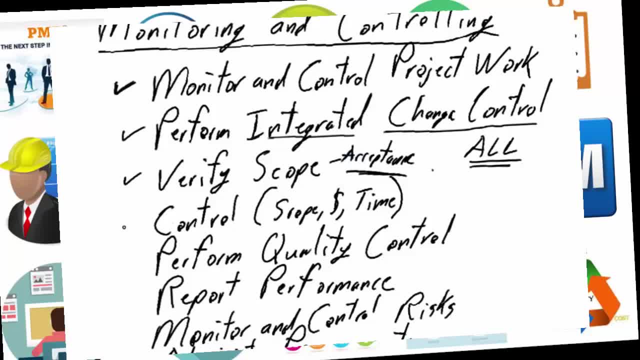 focus is on obtaining final project acceptance. control is what monitoring control is all about: controlling that the scope is appropriate, and we do that through integrated change control, verifying that the budget, that we are still on budget, that we're delivering the project for the amount of money we 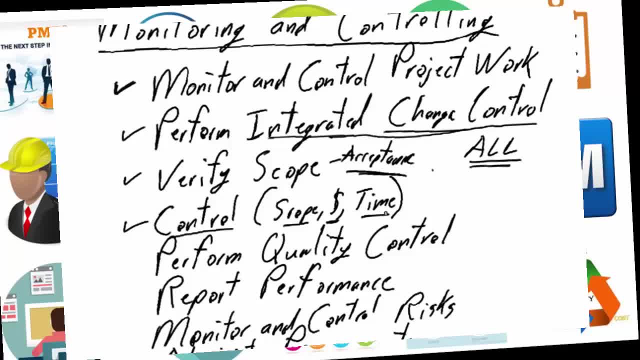 said we're going to deliver it for and that the project remains on schedule, that if this was a six-month project, we are successful, successfully delivering it in six months. we talked about verifying the scope, moving towards acceptance. part of that is performing quality control. are we doing things right in executing? we focused on project quality assurance. are 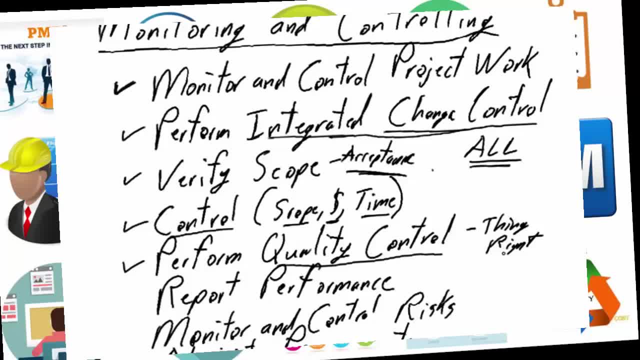 we doing the right things? now we're focused on project quality control. are we doing things right? again, focus is on verifying the scope, moving towards acceptance. we're reporting performance. we're telling everybody how the project is going. we're processing, we're collecting, we're distributing the performance information, the status, the 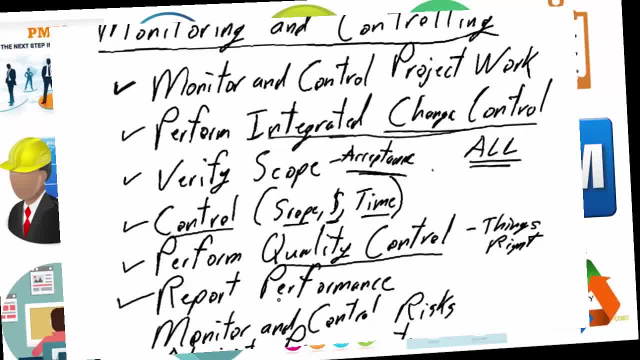 progress measurements and the forecast for the project, and we're going to, through executing, communicate that throughout the world to all of the stakeholders. we're monitoring and controlling risks. we're making sure that we're actively looking at our risk radar and that we're tracking the risk. 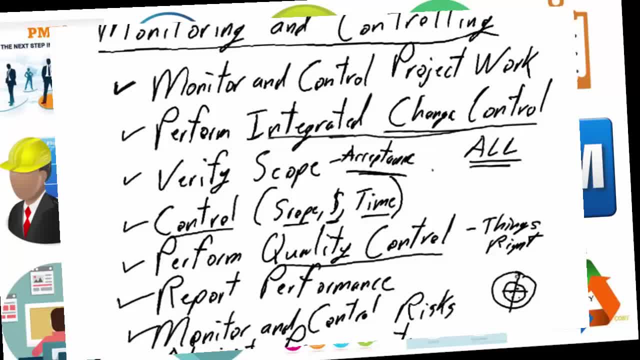 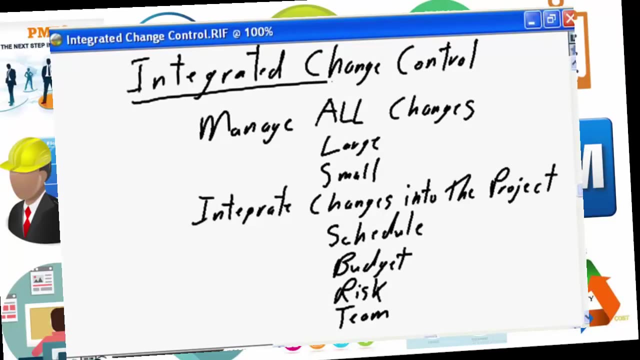 items that are in the focus of our radar, that we're monitoring the further out risks and that we're doing proper risk management. and, finally, we're ensuring contract compliance for all the goods, the services, the products, the raw materials that are being purchased for our project. as just mentioned in the introduction, integrated change control involves 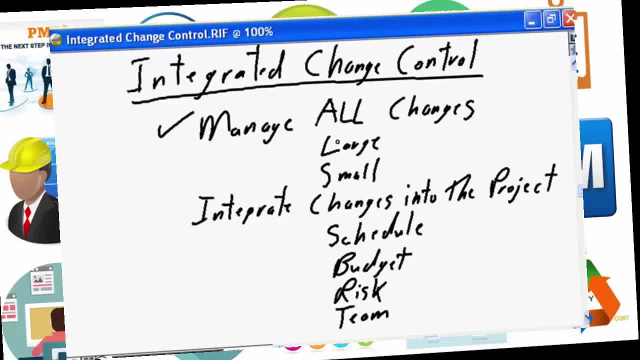 managing all changes, large changes and small changes. large changes need to be managed as separate changes, managed separately, dealt with independently. large changes need to have a separate change document identifying the impact of the change, the ramifications of the change and the approval for the change. so all large changes 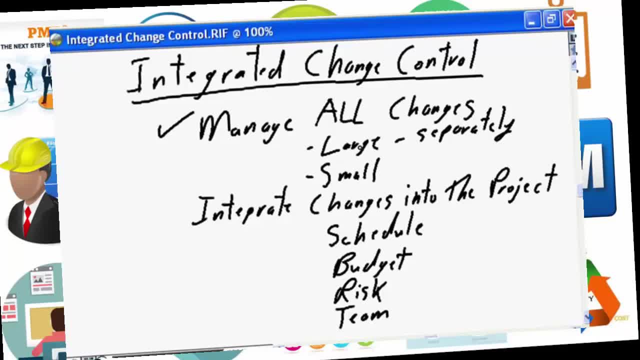 And each project is going to have its own definition of large, but most projects define large as any change involving more than X days. any change involving more than Y dollars is considered to be a large change and it needs to be managed separately: A separate document identifying the impact, the risks and separately approving all large 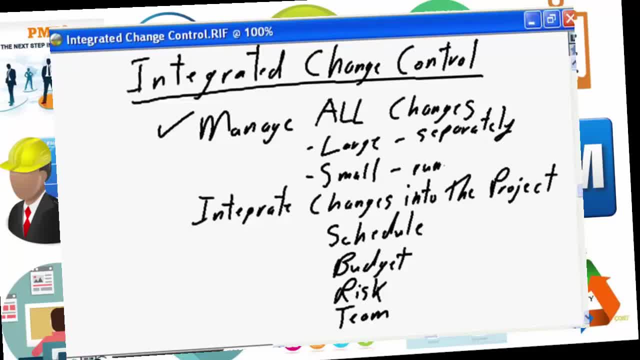 changes. Small changes can be managed with a running change, As we discussed in the detailed review of change management: a running change for this month, for this approved period of time. here are all of the small changes and again small is going to be project specific, but small is all of the changes that don't fall into. 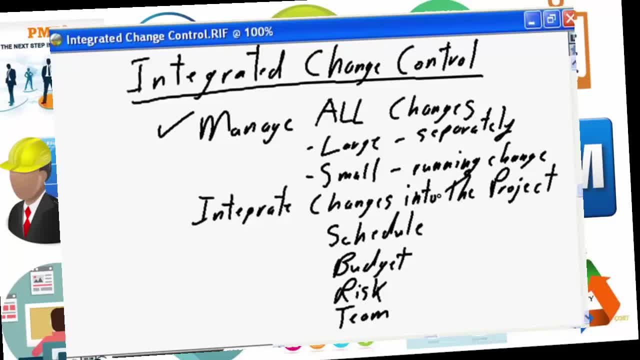 the definition of large. So here are all of the tiny, insignificant changes. We need to change the color from red to green. We need to change the location of the plug from the left to the right. We need to change very minor, may have zero impact on the project budget. may have zero. 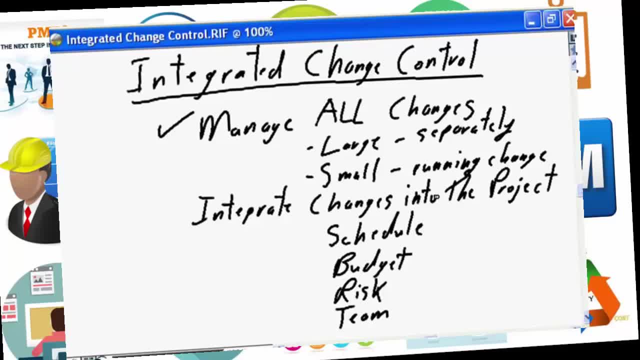 impact on the project schedule but truly have an impact on the final deliverable. It's red versus green. It's managing the expectations, ensuring that everyone is aware that these small changes are taking place, so they are documented and reviewed, and not a surprise at the end of. 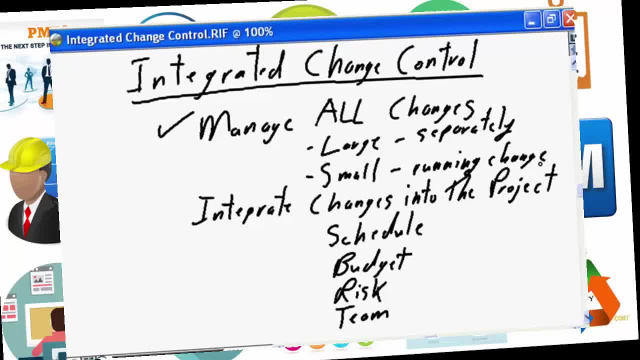 it A running change again. you're going to maintain a spreadsheet, You're going to have a running document that says for this month. here is small change number one, red to blue. Here is small change number two: left to right. 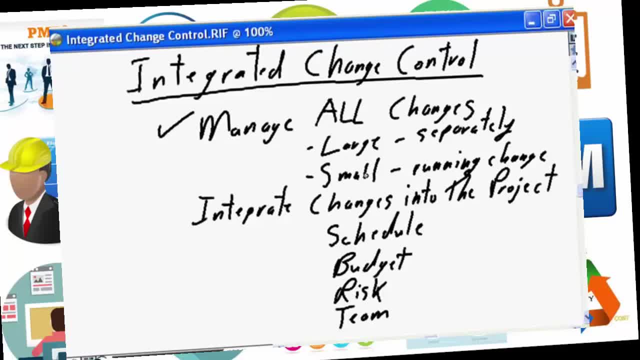 Here is small change number three through small change number 15.. At the end of the period, at the end of the month, all of the small changes would be consolidated and presented as a single larger change for final approval and final acceptance. But all changes. 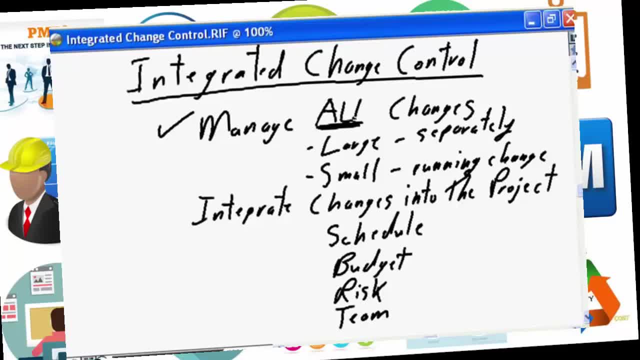 Not some but all changes to any pre-approved, pre-documented project fact- Scope, direction, team quality. any change to any documented fact for the project need to be managed through the integrated change process, And integrated change process says it's integrated into the project. 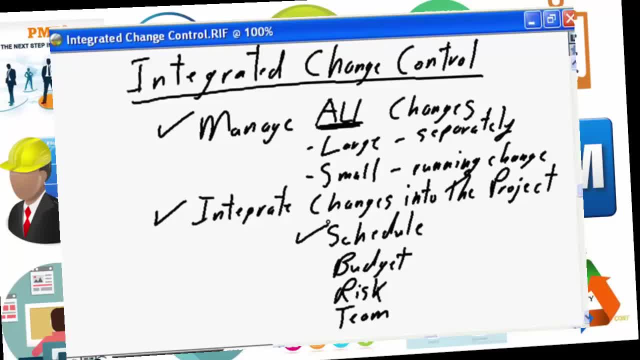 When changes are approved, it must be integrated into the schedule. Tasks must be added to the schedule so that team members can be assigned to work on the change. As tasks are introduced into the schedule, the end date for the project may change. Changes must be integrated into the schedule. 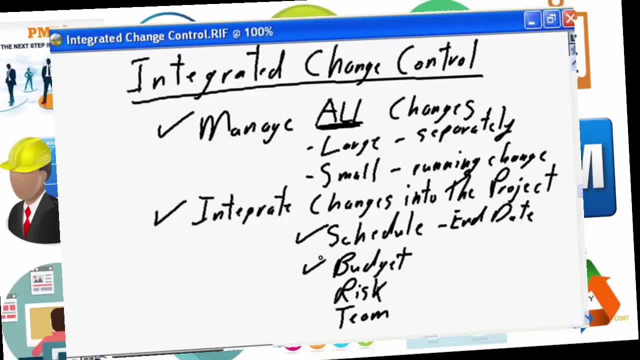 Similarly, as changes are integrated into the schedule, there may be an impact to the budget. It's going to cost more dollars to complete this project as a result of the additional labor that's required to produce the change. Or it may have an impact to the budget simply because additional material, additional supplies must be purchased to satisfy the budget requirements or to satisfy the change requirements. 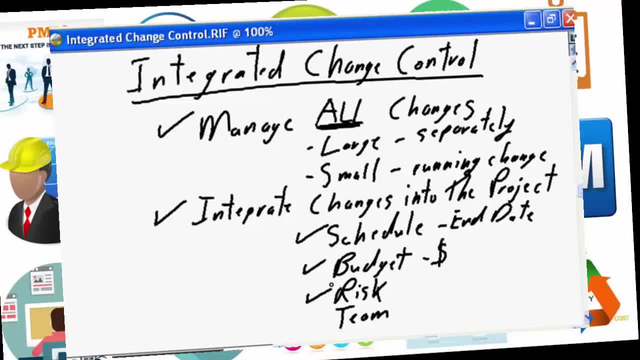 Integrated. in terms of the risk, Does introducing this change to the project add new risks to the project, In which case new risk plans need to be developed. Potentially, additional incremental value for the contingency fund or the reserve needs to be added to the project if the change introduces new risk. 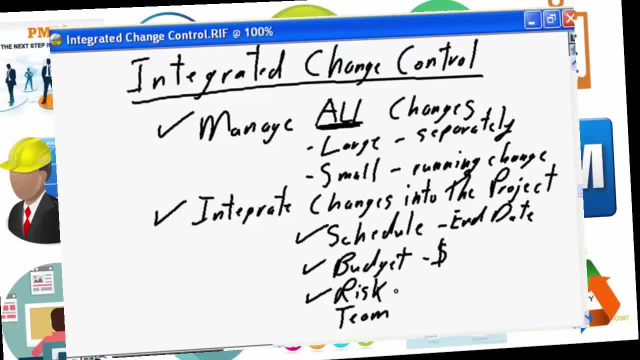 Or potentially, And maybe hopefully, The change is going to lessen the risk for the project. As a result of introducing this change in scope, we've been able to eliminate risk, We've been able to minimize risk impacts Again, in which case the risk contingency, the risk reserve, should be reduced as a result of the change. 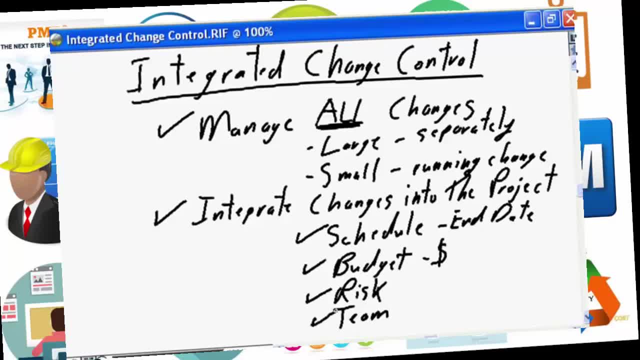 And finally, what impact does the change have on the team? Do we need to change the complement of the team? Do we need to change the skill set for the team? Do we need to add, simply, more team members that have existing skills? So all changes to approved project facts, no matter large or small, develop an effective way for dealing with all changes. 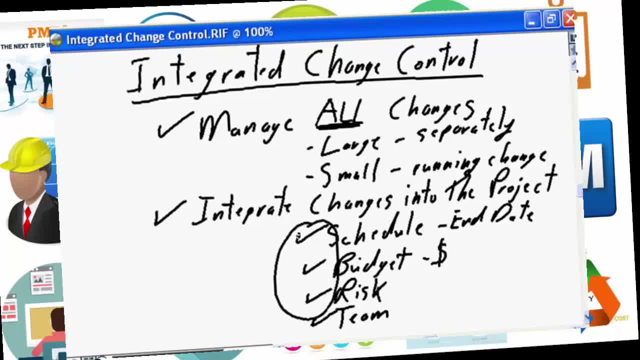 And ensure that all changes are effectively integrated into the total project: The schedule, the budget, the risk, the team, the quality, the procurement, the communications. Every aspect of the project needs to be addressed with the integrated change And addressed as a total project picture, not isolated changes. 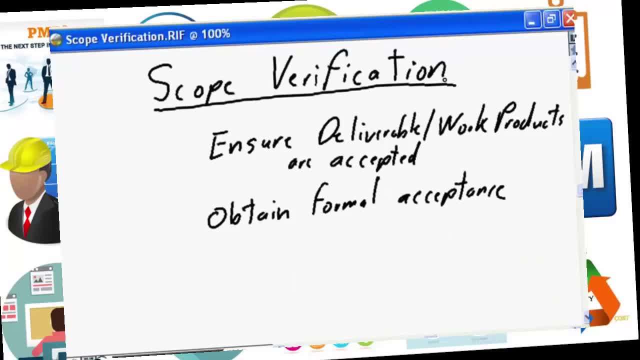 The next step to project monitoring and control is scope verification. Scope verification is not verifying that we're delivering to the scope of the project. That's scope control. Scope verification is ensuring that the deliverables satisfy the scope that final acceptance is going to be approved. 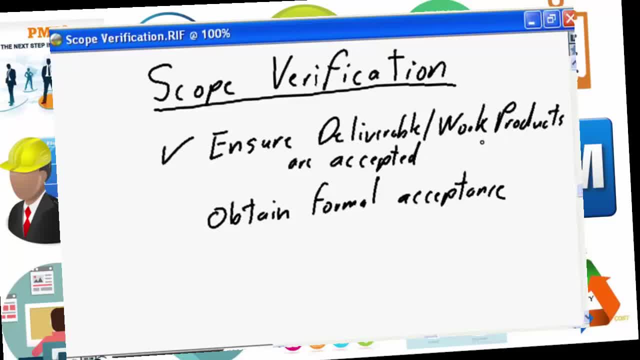 So it's ensuring that each and every work product, each and every deliverable worked on for the project are accepted. It's the ongoing, it's the incremental review, it's the incremental process to ensure that interim deliverables, work in process, is reviewed with the business unit to ensure that, yes, this work being produced satisfies our expectations. 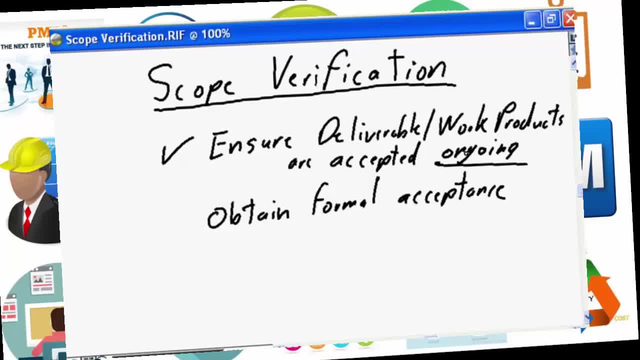 Ensuring that the end product, when it is finally delivered, will satisfy total project requirements. So, if you do good, scope verification, ensuring that all interim, all work in process is reviewed on an ongoing basis. obtaining the formal acceptance when the final deliverable is presented to the business for formal final acceptance. 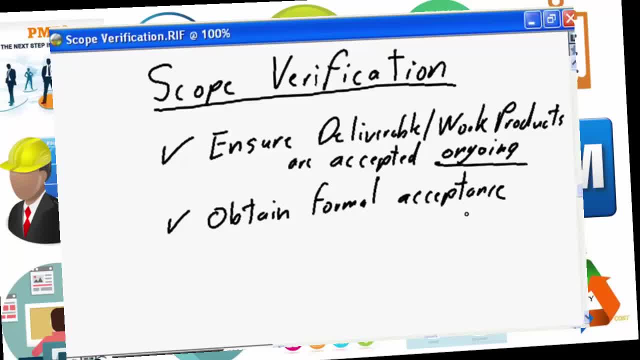 it should be a routine matter of the fact. of course we're going to approve your project deliverable. Of course we're going to sign off your project. We've seen every piece of work that the project has completed to date and there's absolutely no reason why. 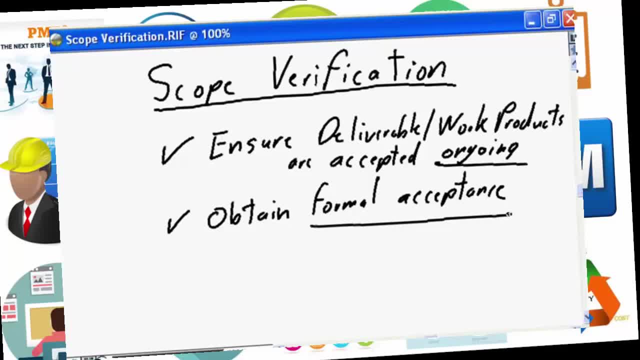 I wouldn't be happy to give you formal acceptance. Ongoing scope monitoring and control, in terms of the scope verification process, the interim review, the ongoing activities, ensures that final acceptance of the process, final acceptance of the project deliverables, final acceptance of the project itself. 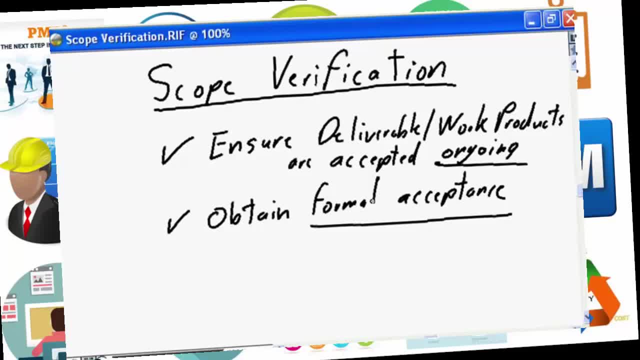 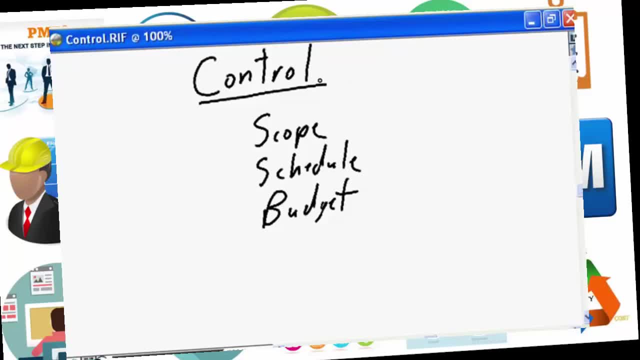 will happen in a timely, efficient fashion. As indicated by the title for this project management process, we need to ensure we have total control- yes, I believe total control- over the project. As a project manager, we need to ensure we have absolute understanding of the scope. 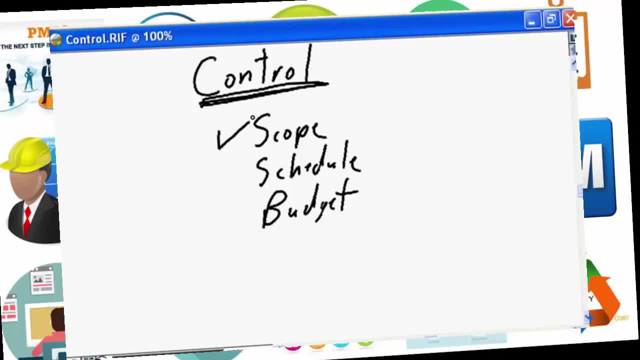 Is the team delivering? is the team working on the tasks? are the deliverables being produced by the team satisfying all of the scope requirements and only the scope requirements? We want to ensure there's no gold plating. we want to ensure there's no embellishment. 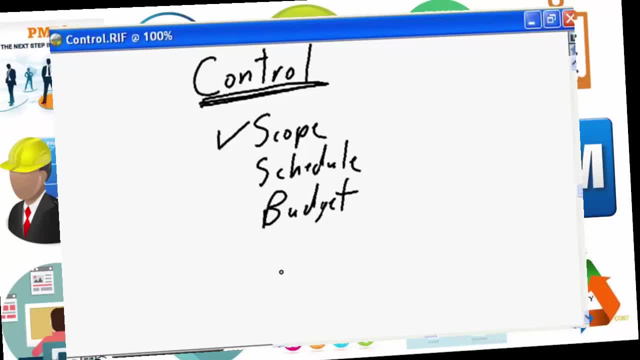 that we are delivering exactly what the scope specifications are going to be. We need to have an ongoing understanding of how the team is doing For each and every task that the team is working on. is the task being produced according to original schedule? Is the team spending more time, more effort on a task? 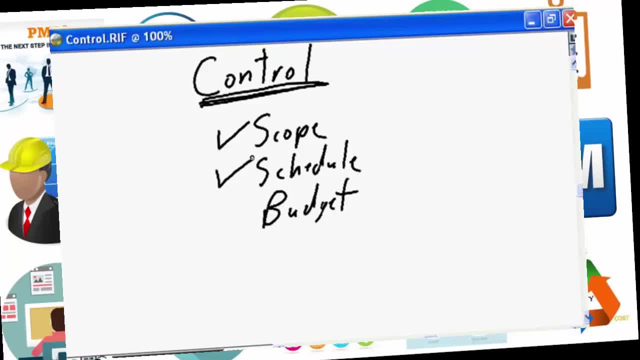 Is the team spending less time, less effort, on the task. We're going to effectively monitor and manage our critical path for the project, ensuring that any variations as the team is working on individual tasks we can reflect and understand the impact it's going to have on the total project schedule. 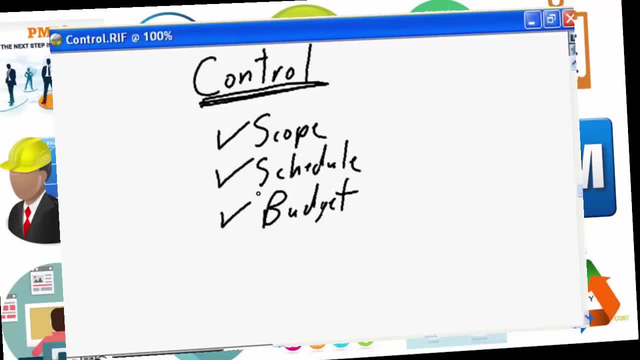 and the component of control that is probably most carefully monitored in all organizations is the budget. Budget dollars are very easily understood by everyone. Everyone in the business understands the impact of spending dollars on a project. It's dollars that's not available for company profitability. 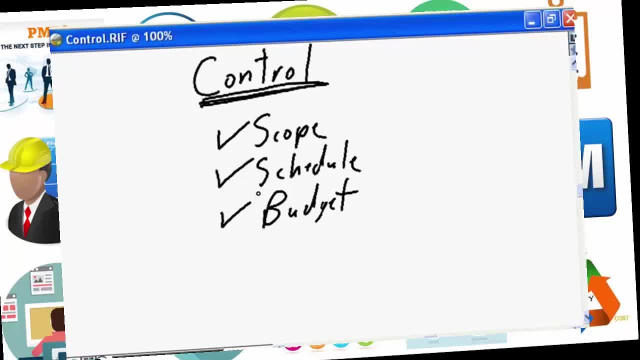 or it's dollars that's not available to be spent on other activities in the project. So, as a project manager, we need to carefully, diligently monitor the scope, the schedule, the budget. We need to be prepared to work and rework. 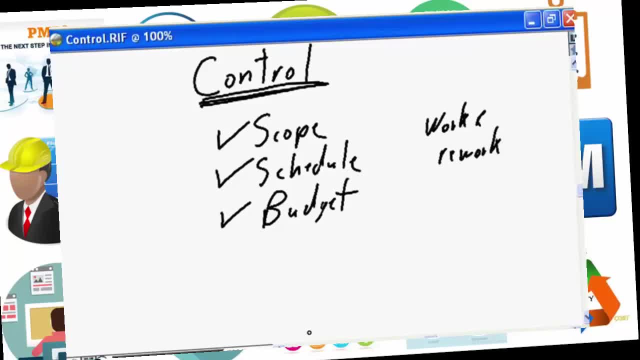 The schedule, the scope, The budget On a weekly basis. So every week we need to understand: is the project on scope? Are we delivering the right tasks? Is the team delivering the work according to schedule? What impact does Johnny spending six hours more on a task? 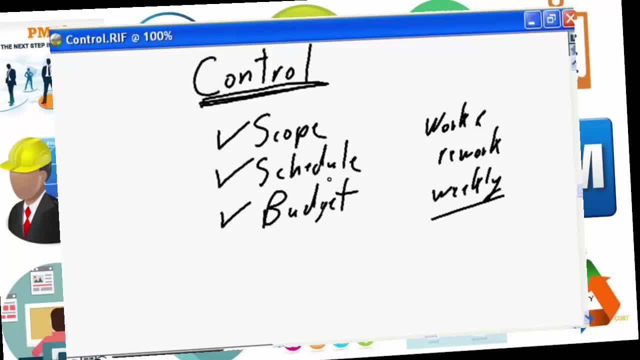 what impact does Mary spending three hours less on a task have to the total project schedule? Are they on the critical path? Do we have slack? What impact? What impact is this going to have on the project end date? Do we need to notify the business that the project is going to be late or early? 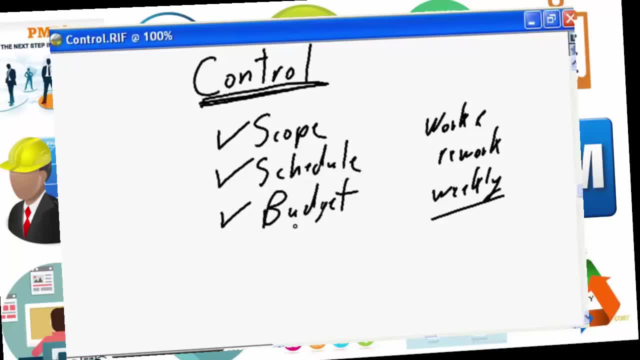 What impact does the actual work being done on the project have on the overall budget Based on the facts, just the facts, ma'am, just the facts. on the work that is done for the project, you, as a project manager, will be working and reworking the scope, the schedule, the budget. 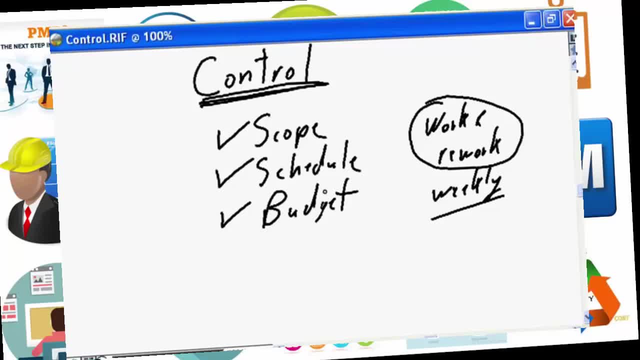 realizing that we have the triple constraints, that if there's a change to one of these components, the project is going to deliver more or less scope. it's going to have an impact on the schedule. the project is going to take more time to deliver more scope. 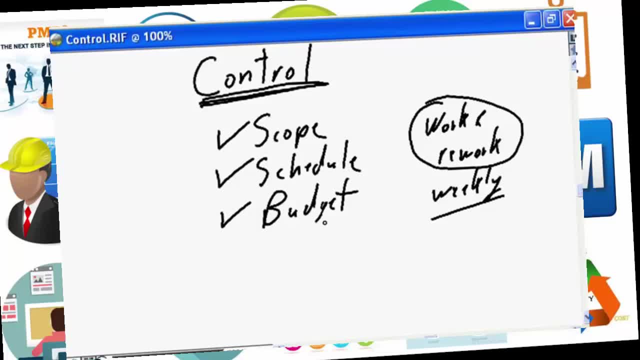 or the project is going to take more budget, more dollars to deliver more scope. So we need to work and rework this from a project management viewpoint to ensure that the facts, the actual details we have from project delivery, from our team members- and we're going to do this on a weekly basis- 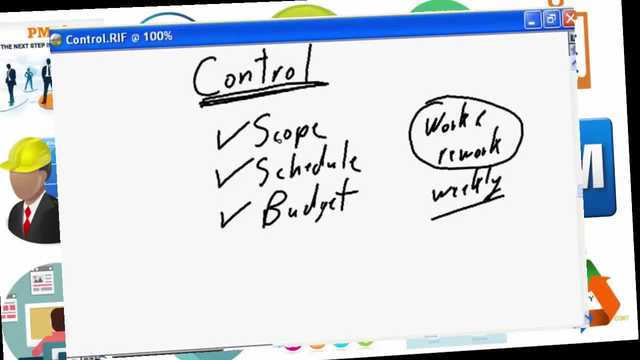 that we have firm control over the project And we develop and understand that firm control, because we're going to control it, we're going to manage it, we're going to work against our project. baseline- The original statement of the scope. it's going to look like this: 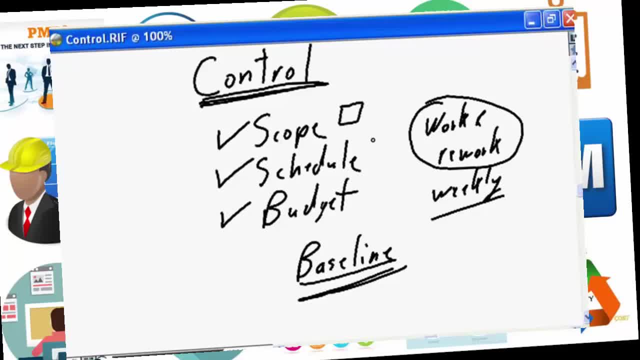 it's going to be a blue box. The original definition of the schedule. it's going to deliver on August the 23rd. The original definition of the budget. it's going to cost $50,000 to deliver the project. That is our baseline. 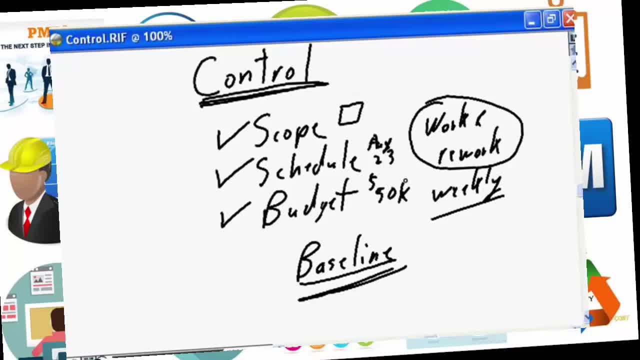 This is what the scope looks like. this is the original project end date. this is the original project budget, As we get the facts on a weekly basis from our team. we're going to work and rework. we're going to understand the triple constraints. 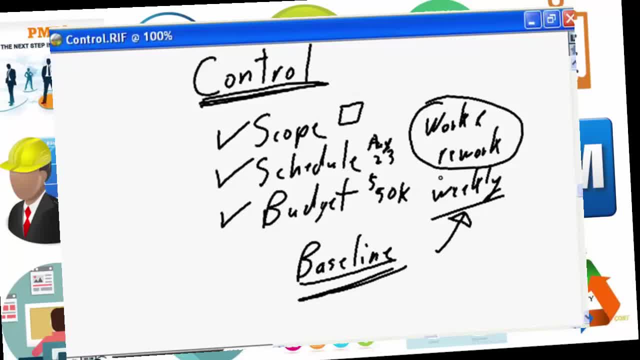 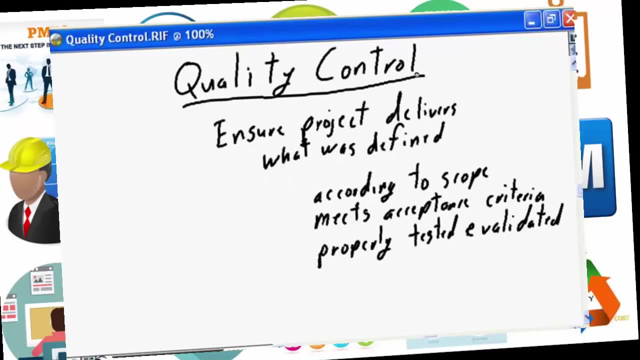 the relationship between scope, schedule and budget and we're going to monitor and rework that against our project baseline and work with our project sponsor to make any revisions necessary to satisfy the overall business requirements. An additional control element- quality control- is part of overall project monitoring and control. 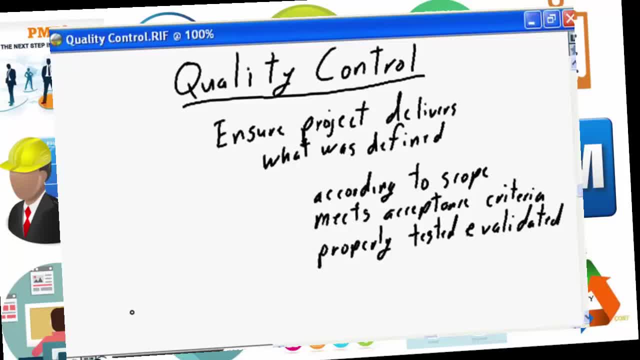 Quality control ensures that the project delivers what was defined, that the end product, that each end product, that all work products produced by the product satisfy the overall business requirements, ie, that it is delivered according to the scope. We want to ensure that each end product. 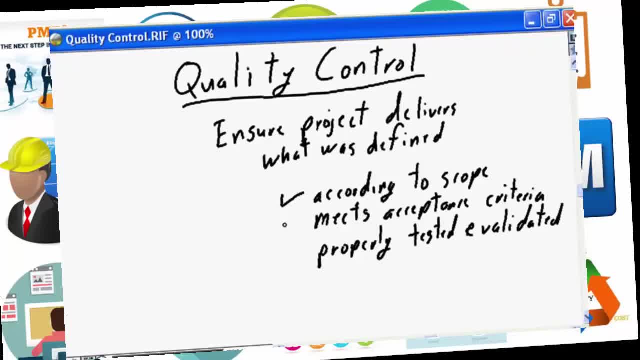 that each product, each work product, meets the scope and therefore will meet the acceptance criteria. The only way to ensure that all of the products produced by the product are going to address the scope and meet the acceptance criteria is to ensure that they're properly tested and evaluated. 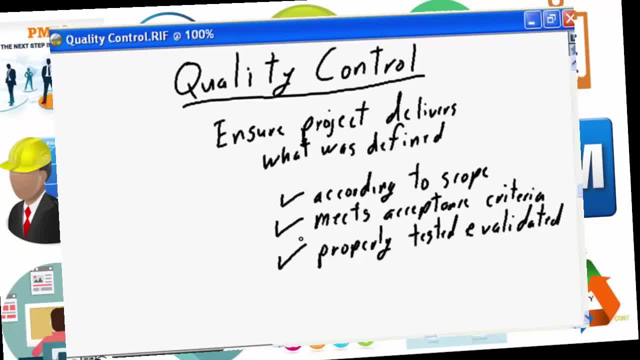 that each component has been reviewed internally within the team, been through the proper review processes, the walkthroughs and validation processes to ensure that each deliverable is produced according to scope, that it's going to satisfy the business criteria, and it's the team's responsibility to review, test and validate. 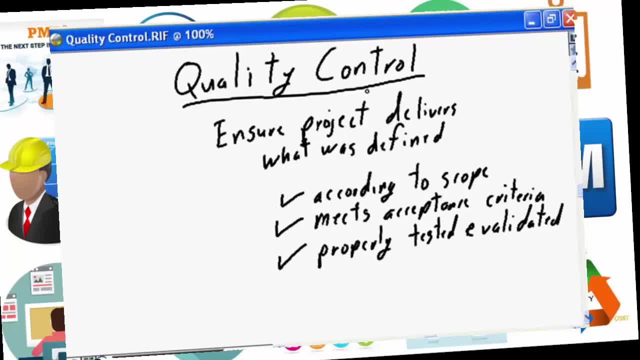 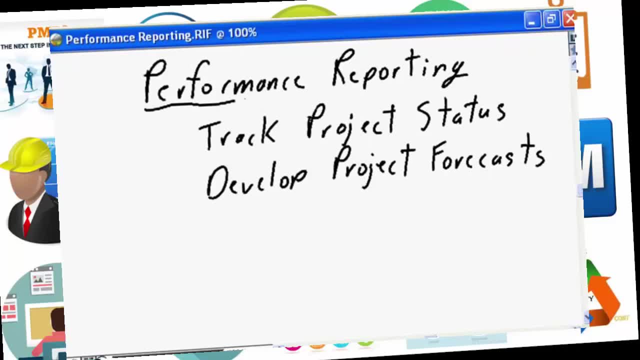 to ensure that, again, the quality control processes are being followed and that the project delivered exactly what was defined. The next step in project monitoring and control is performance reporting, Gathering and consolidating all of the actual details, the status reports from the team members. 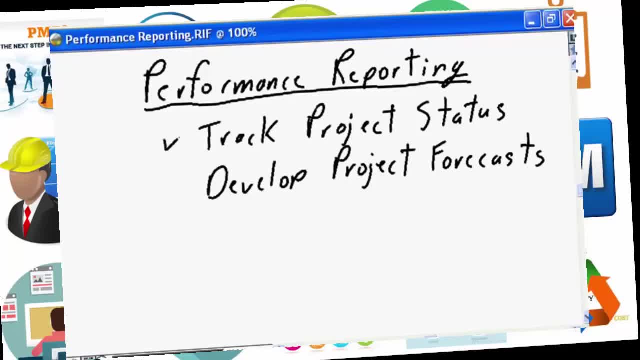 so that you can communicate that information to the appropriate stakeholders in the organization. So it's tracking project status. We've already received detailed status reports from each and every team member. Team member number one worked on task A, B, C, D, E. 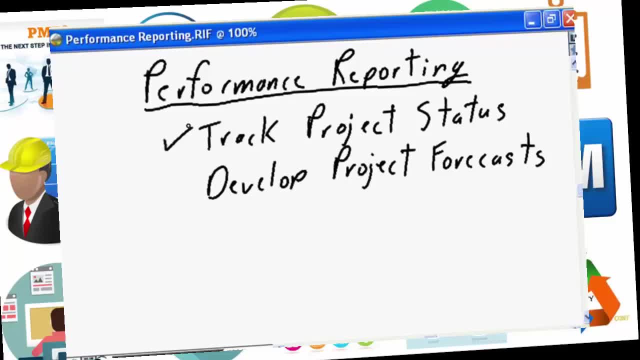 Team number two worked on tasks M, N, O and P. It's consolidating all of the detailed project status information from each and every team member. consolidating bringing it up to the appropriate level of summary information because typically a project status report. 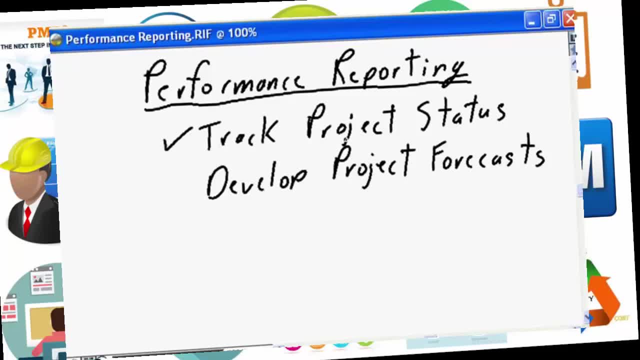 is not going to have information at the task A, B, C, D. It's going to have information at the summary level A and the summary level M to provide the status information to your project sponsor and maybe even at a higher level of summary detail. 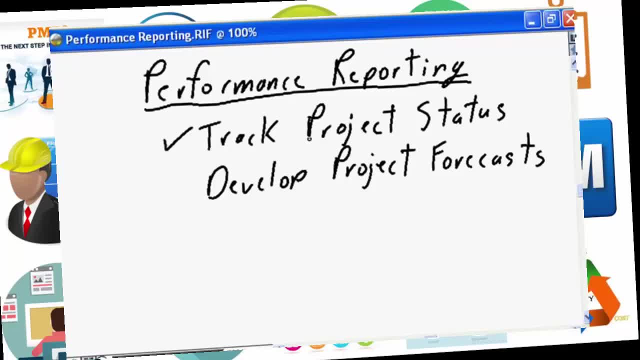 for communications to higher level management in the organization. So it's tracking and consolidating the detailed project status from each team member to produce the appropriate status information, the appropriate project performance information for reporting to higher levels in the organization, to all of your project stakeholders. 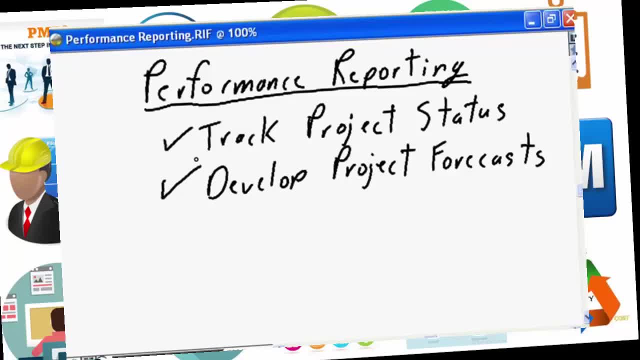 Once you have detailed project status in place, it's important that you develop the project forecasts. In the control section we discussed how you need to work and rework the schedule Based on the facts that you now have from your team members. I am forecasting that the project 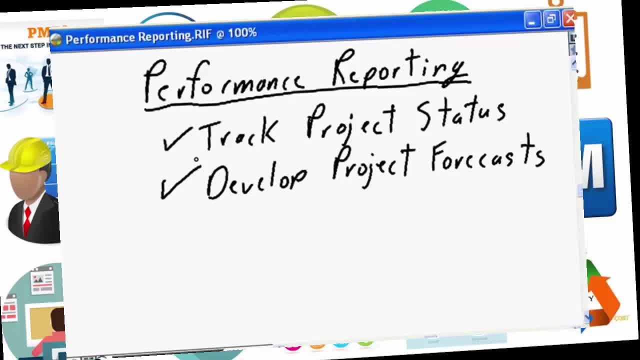 will now cost an additional $200,000, $2,000, $20,000.. Based on the status information I have from my team members, I am now predicting that the project will be two days late, three days late, two weeks late. 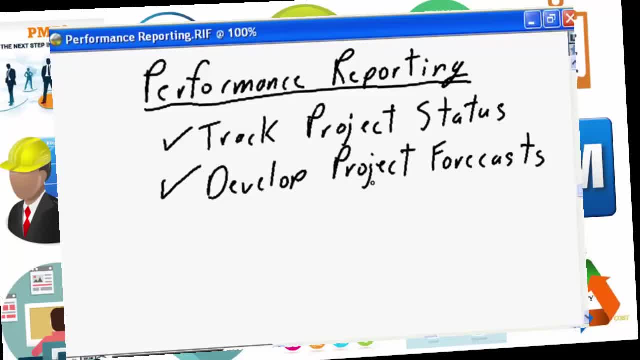 It's developing the revised forecasts based on the facts that you have at hand from the detailed status reports that you have gathered and summarized as part of overall project performance reporting. It's to develop a new picture of where the project is now and what is the new completion. 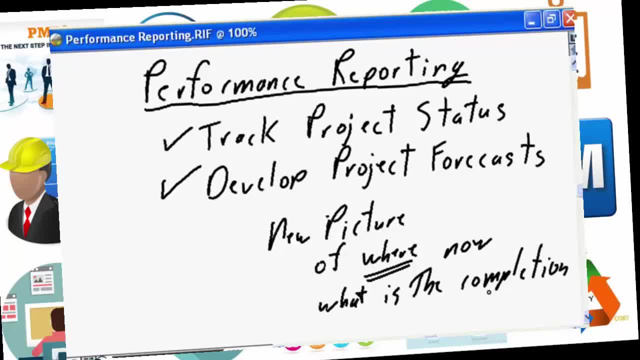 Based on the information I have at hand, based on the project forecasts. this is now how I am forecasting my project will complete, And when completion forecasts begins to look significantly different than the original project baseline, it's time for you to work with your project sponsor. 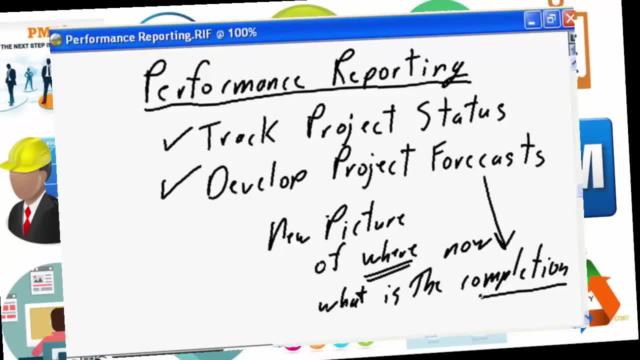 to take the appropriate actions based on the triple constraints of scope, time and cost. What can be changed to allow you to improve the completion picture, Assuming again that, on average, projects complete later and over budget as opposed to earlier and ahead of budget? 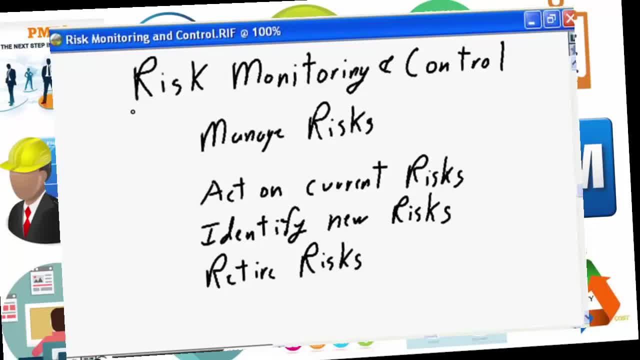 The most important aspect of project monitoring and control is risk monitoring control, At least in my humble opinion. risk monitoring control, risk management- is the single most important thing that you, as a project manager, can do to ensure your project is going to deliver on time and on budget. 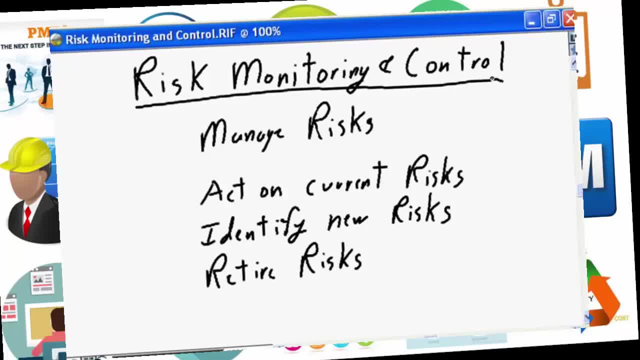 Risk management is where we're going to deal with the unknowns. we're going to try to proactively eliminate, minimize the unknown problems that can happen on our project. that's going to cause challenges. that's going to cause it to deliver late. 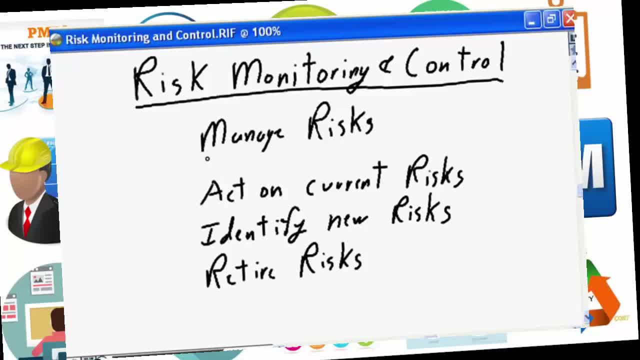 that's going to cause it to be late. We need to effectively manage all of the risks and instead of managing, maybe the best term is we want to, where possible, avoid risks Because they're unknowns. some risks are going to be unavoidable. 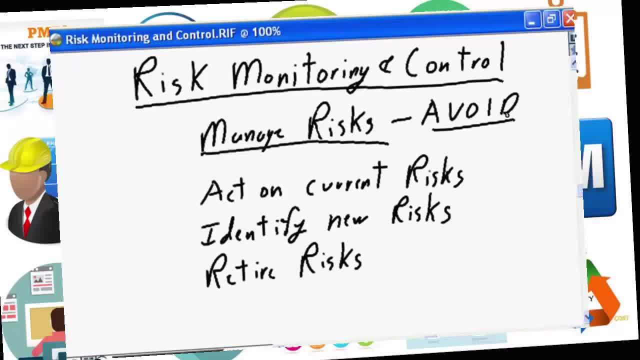 Some risks are also unmanageable. There is nothing you can do about the weather. If weather is going to cause you or your project to have problems, if, as a result of weather, there will be days your project cannot be worked on, there's very little you can do. 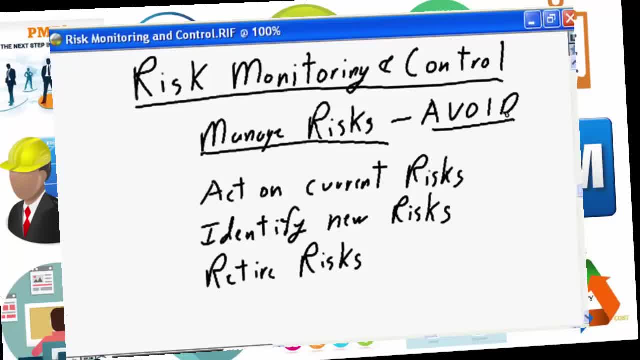 to eliminate the risk of bad weather, But we need to manage the risks. we need to avoid the risks. we need to ensure we're taking actions to deal with the risks. In order to do that, we need to act on the current risks. 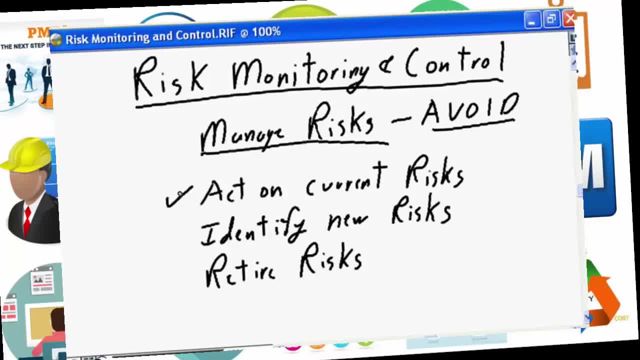 During project planning, we developed a list of all possible risks that could possibly impact our project. We then categorized and prioritized the risks and came up with the truly serious risks that we need to manage on their project. We then put them into a detailed timeline. 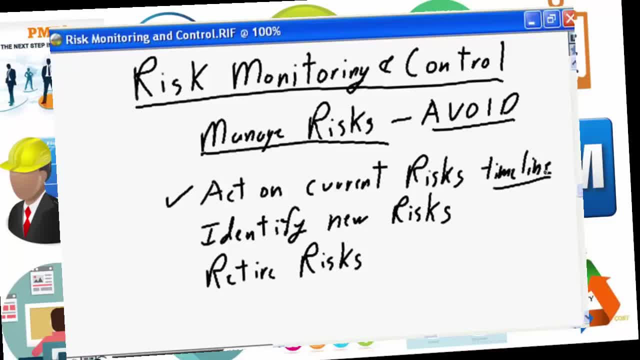 to determine when, on the project, the risks could possibly come to fruition During project delivery, project monitoring, control. we need to be acting on the current risks, based on the timeline of when the risk is likely to impact our project. We need to now understand. 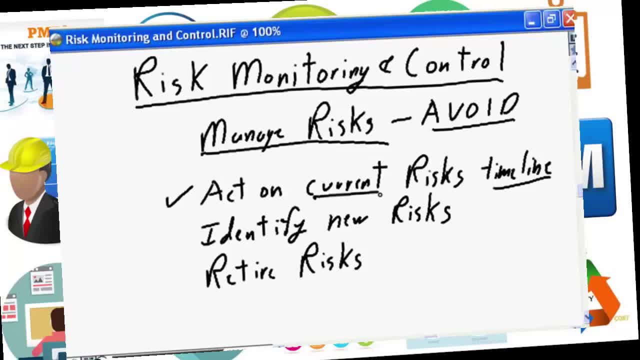 what risks are possibly going to impact our project at this moment and over the next near future, the next few weeks, maybe even the next month or the next two months. We need to be taking our actions now on the current risks, to manage them, to avoid them. 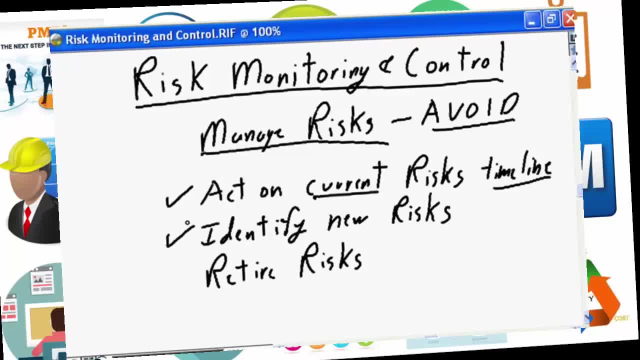 to eliminate, to keep them from happening At the same time, on the outlook for new risks As a result of the project progressing to this point in time, have new risks been identified As a result of more information? as a result of potentially changes? 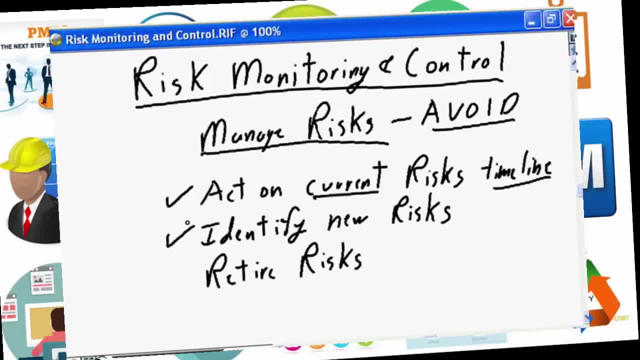 to the project integrated change management. have new risks been identified? What actions do we need to take to deal with these new risks? How are we going to manage, how are we going to avoid the new risks? Again, eliminate the risks. 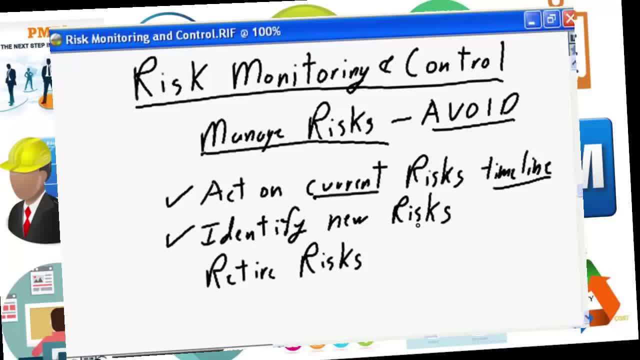 put plans and strategies in place to keep these bad unknowns from impacting your project. And the thing I enjoy most about risk monitoring and control is retiring of risks. I had a risk that my team was going to require training As a result of the work. the team 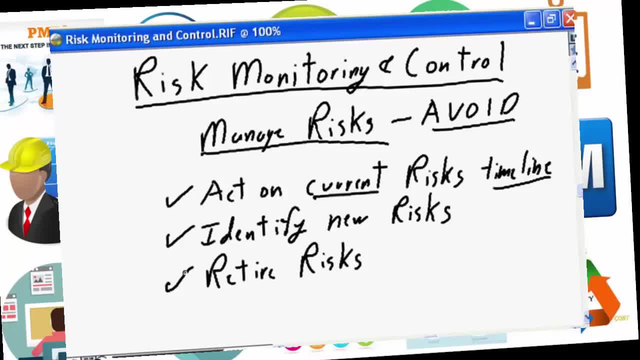 is now performing on the project. I realize they have all of the skills they need to complete their tasks. The risk for training can be retired. It is no longer a risk for the project. There's one less thing that's going to keep me awake at night. 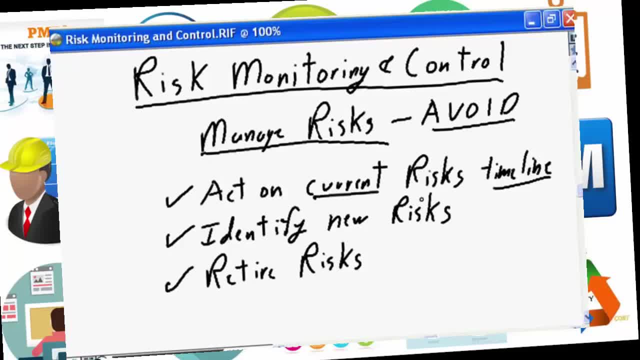 So when we're managing risks, when we're acting on the current risks, we're identifying the new risks and we're retiring risks. we're dealing with the part of our project called contingency, Or another term for it is often reserve, As we're in risk monitoring and control. 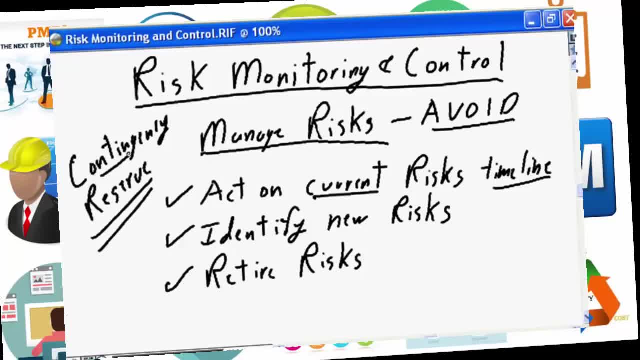 we are using up, we are consuming our contingency, we're consuming our reserve. So for risk number one, we had a contingency of five days and five thousand dollars. We're acting on the risk. we've determined that, yes, risk number one is truly going to impact. 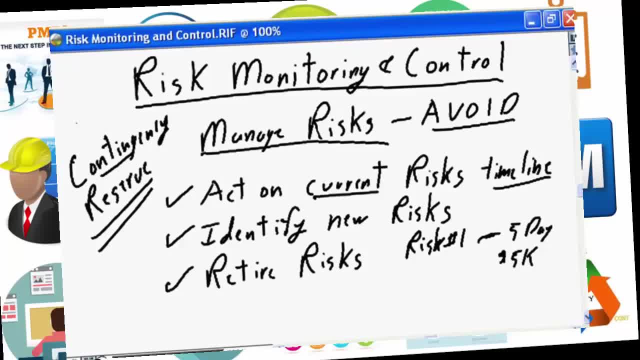 our project at this point in time. therefore, we're going to go to our contingency and we're going to remove five days and five thousand dollars from the overall contingency fund to take the actions, to give us the schedule relief, to give us the budget relief. 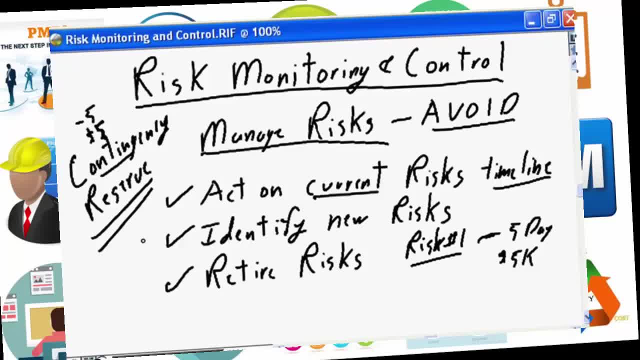 as a result of risk number one transpiring into our project. The same thing: when we're retiring risks, we realize that risk number six, which had a two day and, for simplicity, two thousand dollar contingency reserve and typically a risk, is not going to have. 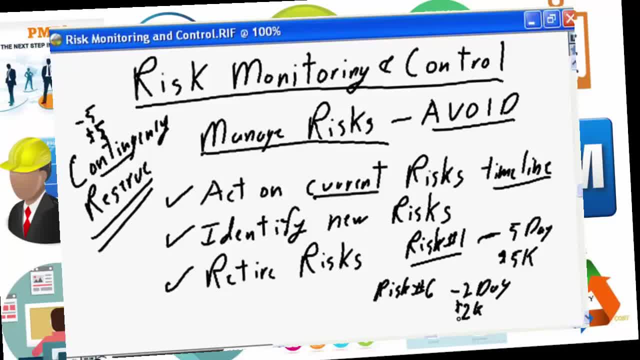 a direct correlation between days and dollars, but for simplicity I'm using the terms this way. risk number six is being retired. it's not going to happen. any issues on our team is not going to happen. so therefore we know we have extra. 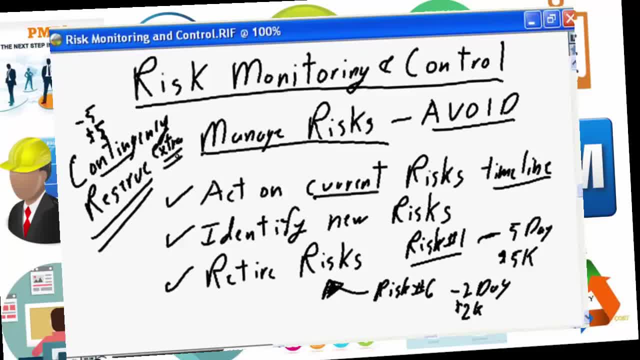 contingency, extra reserve on our project that we can use to deal with the new risks, that we can accept new risks into our project without having to go back to management for additional contingency and additional reserve, because we have the additional contingency and reserve as a result of retiring risks. 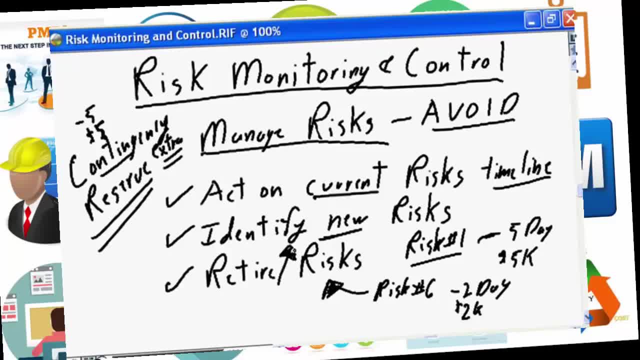 Risk monitoring and control, in my humble opinion again, is probably the hardest aspect of project management to grasp, because you're dealing with unknowns, You're putting together funds, you're putting together plans, you're putting together schedule relief for a series of 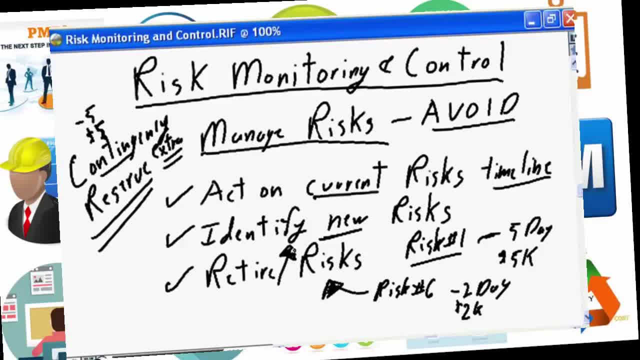 unknown events that may or may not happen in the future. But without proper risk management and control, risk monitoring and control, without proper management and allocation of contingency and reserve in your project, you will have no recourse when bad things happen to your project. 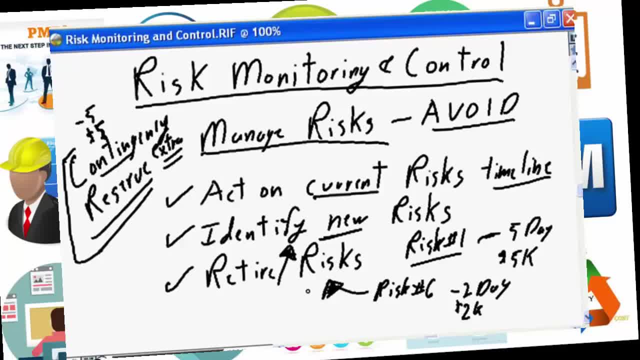 unplanned bad things happen to your project, The only recourse you would have, without proper risk management, is say: the project is late, the project is over budget. With good, effective risk management, we simply begin to consume. we remove the time, the dollars for risk number one from our contingency. 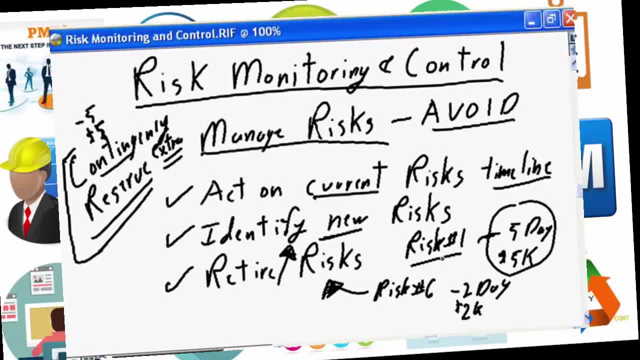 and we're still able to report risk has happened. a bad thing has happened on my project, but because of effective risk management, the project is still on track. That's what project management, risk monitoring and control is all about. The final aspect of project monitoring: 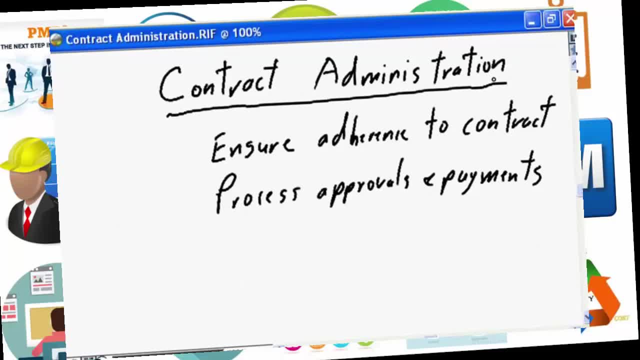 and control is contract administration: Ensuring that all contracts, all purchases that your project is making, that your project requires, are properly managed and administered. It's ensuring adherence to the contract. And when I say ensuring adherence to the contract, I'm talking on both sides. 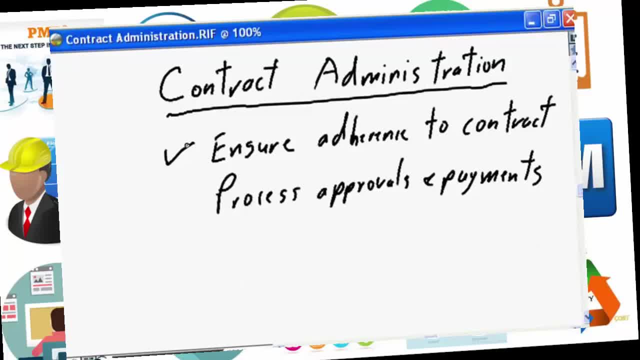 of the contract. Contracts are two-sided, hopefully- fair documents. Your sellers, your vendors, have certain obligations to you under the terms of the contract. You will manage to ensure that your sellers are delivering what it is your project requires, in accordance to the 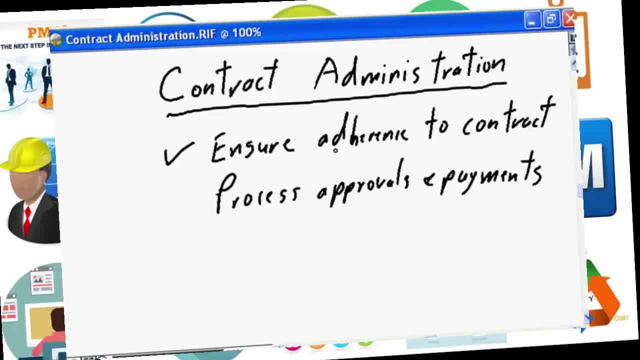 terms and conditions of the contract. Similarly, your company has certain obligations back to the vendors. Obviously, they are going to expect payments, but they may be also expecting feedback, turnaround supplies, access to intellectual property, access to specialized equipment that your organization has in order. 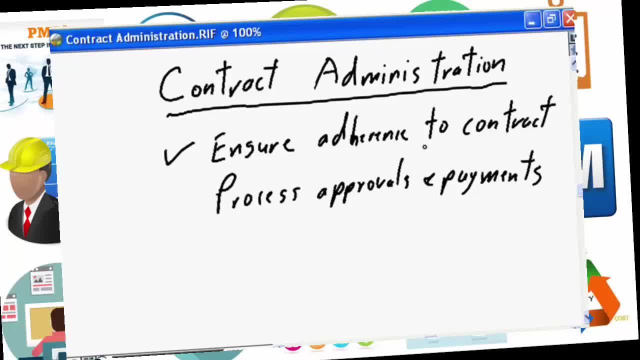 for them to fulfill their side to the contract. So you need to ensure adherence to both sides of the contract. You can't treat contract administration as purely a one-sided street, one-way street, where the only issues are you making sure you get everything you need. 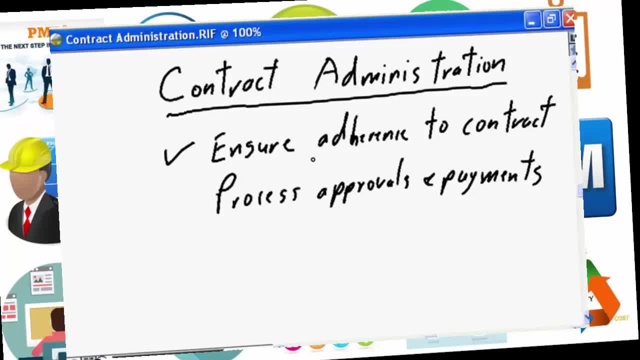 out of your vendors. Obviously, you want to do that, but you also need to ensure that you are supplying the support to your vendors that they need to deliver the goods, the services that you need for your project. The next aspect is, obviously, your vendors are going. 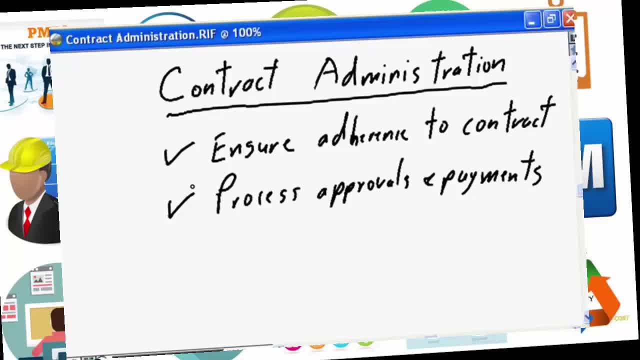 to want to be paid. So you, as a project manager, will work with your procurement department to ensure proper processing, prompt processing of payments, that you are giving your vendors the proper approvals that they need to allow them to continue to execute on the project Effectively. 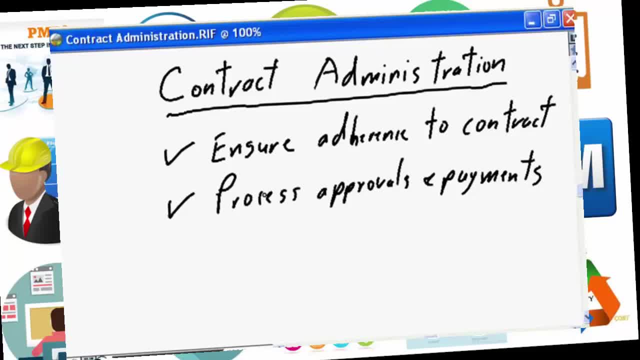 with contracting administration. you have become the customer. you are effectively the project sponsor. you are effectively the acceptor for the components of the project that your vendors are delivering. So you are delivering administering managing contracts as a mini-project within your total project, where you 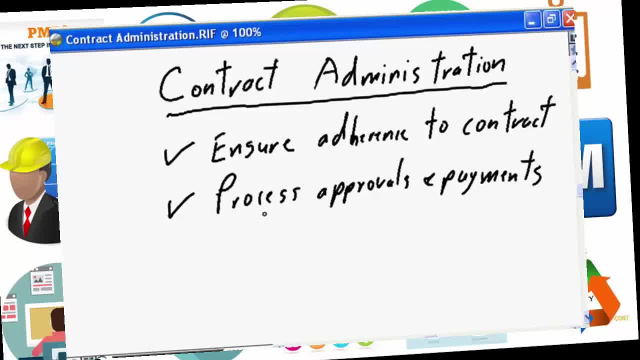 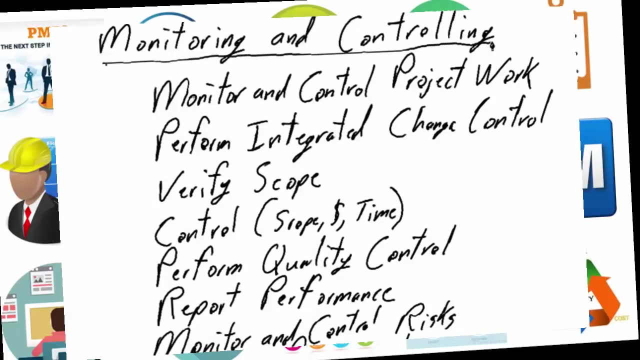 have switched hats: Instead of being the deliverer to the business through contract administration, you have become the acceptor, the sponsor for the components to the project that are being delivered by your vendors. This concludes our fourth nugget on the five process groups, This one on monitoring and control. 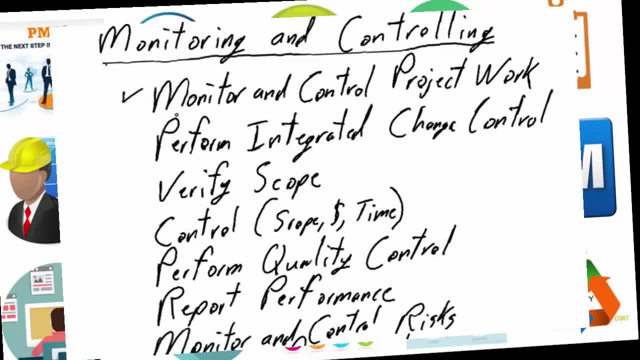 As the first bullet says, monitoring and controlling is where we, the project managers, monitor and control all of the work: making sure that the project remains on schedule, make sure that all of the work that our team members are doing in the previous process- group executing- are focused. 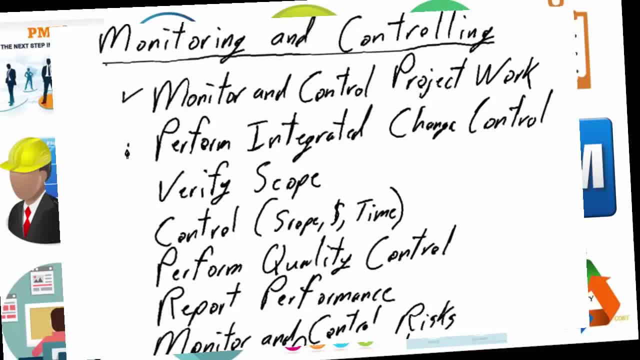 on successful conclusion. Monitoring and control is performed through integrated change control, making sure that all changes, every change to the project, is processed through change control and, more importantly, that the change control is integrated, that all changes consider the impact on cost, time, scope. 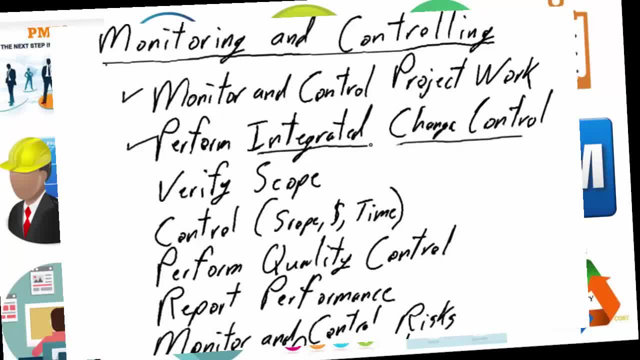 quality, human resources procurement, etc. etc. through each of the nine knowledge areas. Integrated change control is what we need to do as project managers to ensure that we do all of the work, and only the work that is required for the project. 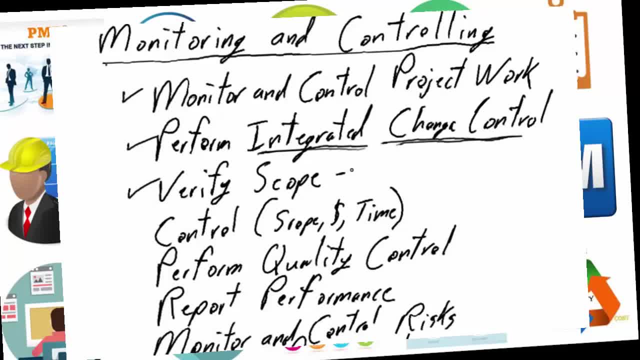 Monitoring and control is all about verifying scope, moving towards acceptance, Making sure that each deliverable in our project is oriented towards final project completion and that each deliverable we produce for the project has the appropriate components in it to ensure that the deliverable itself gets accepted. 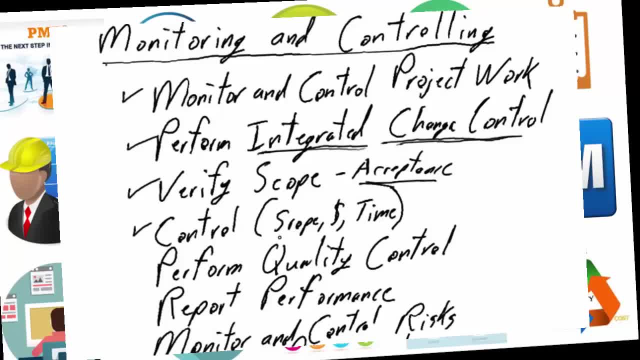 Monitoring and controlling obviously is all about control. We're going to control the scope of the project. we're going to ensure we do all of the work and only the work, and that's largely done through integrated change control. We're going to control the project's. 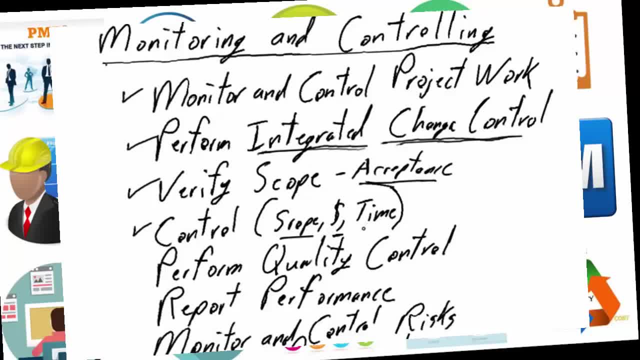 budget to make sure that our project is delivering on budget and that the project is delivering on time. Quality control is going to make sure we're doing the right things. We're going to ensure that the appropriate quality control activities are taking place to ensure that the right things are being. 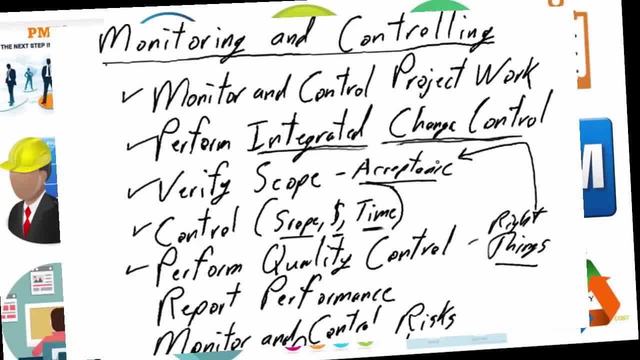 done that. the work is being done focused on project acceptance. We're going to track and manage and report on project performance. We're going to understand and report on the project status. We're going to monitor and control the risks. We're going to 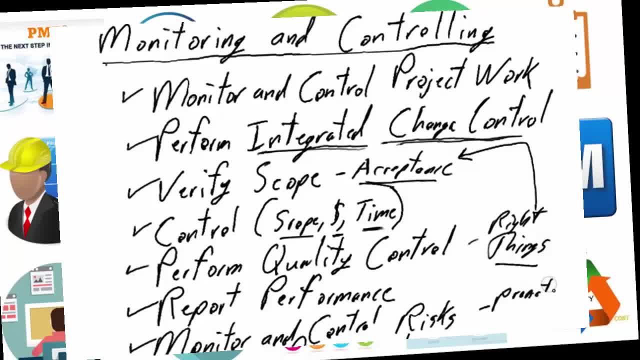 take proactive actions to reduce, to minimize, to prevent unknown bad things from happening on our project. And finally, we're going to administer procurement, We're going to manage the contracts. A couple of notes to wrap up: monitoring and control. One of them is: 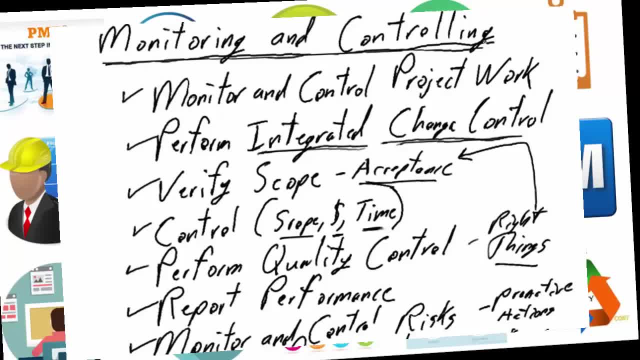 there are two less processes in monitoring and control in the fourth edition of the PMBOK from the previous edition. Two processes, one being manage project team and the other being manage stakeholders, have moved from monitoring and control and are now part of executing, as we discussed in the 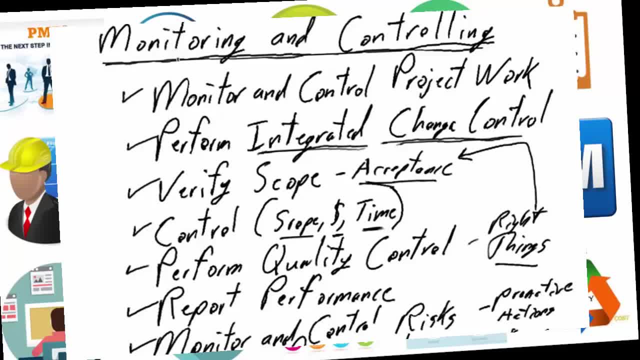 previous nugget. The other note is: throughout this nugget I left some of the PMBOK release three terms in the detailed parts of this nugget. For example, the last component we just talked about in PMBOK release four, it's called administer procurements. 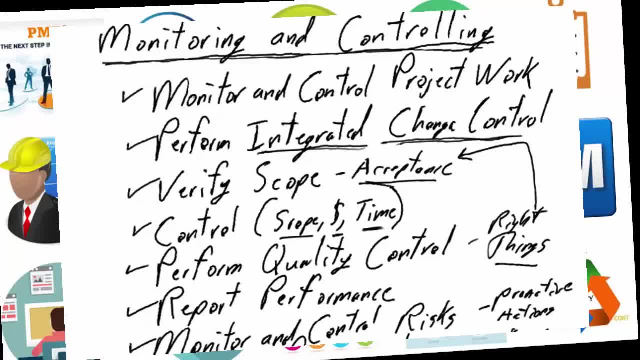 The rename again is largely based on the noun verb process. In the previous release that was called contract administration. So again there were subtle variations on some of the names in the detailed versus today's names in the PMBOK guide. Doesn't impact.